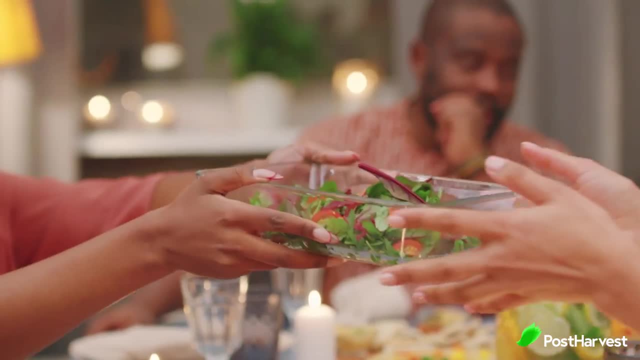 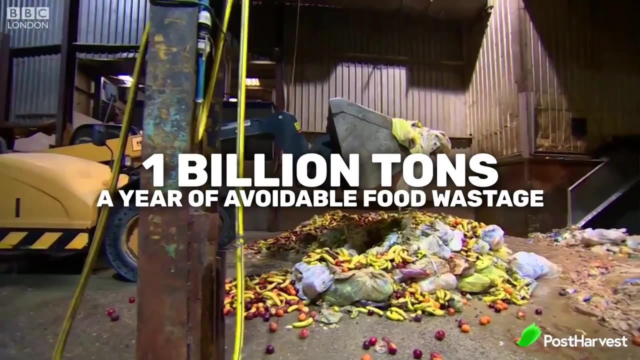 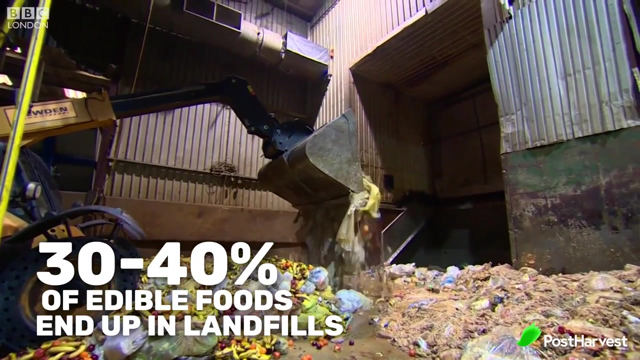 half thousand each year. Think about how many more meals that equals up to Number seven. there are about 1 billion tons a year of avoidable food wastage from production to consumer stages. This means 30 to 40 percent or more edible foods end up in landfill instead of on the plates. 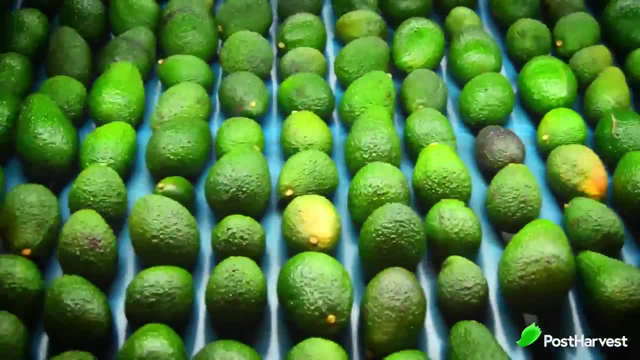 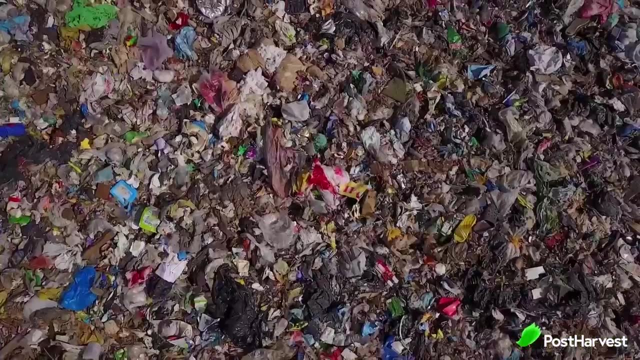 around the world. Number eight: if everyone ate one less serving a day- a banana here, half an avocado there- we could save 10 million metric tons annually. Number nine: eliminating global food waste would save 4.4 million tons of CO2 a year. 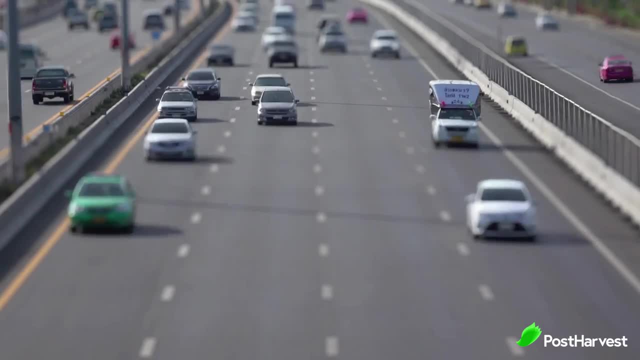 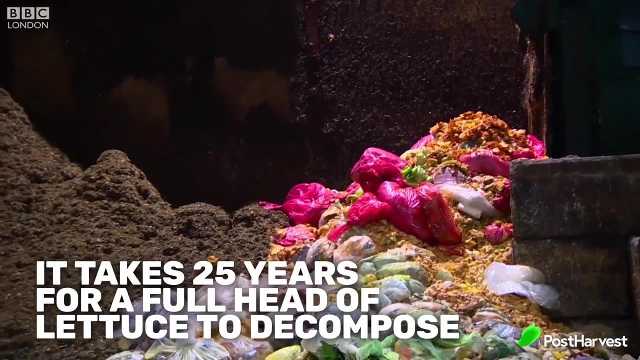 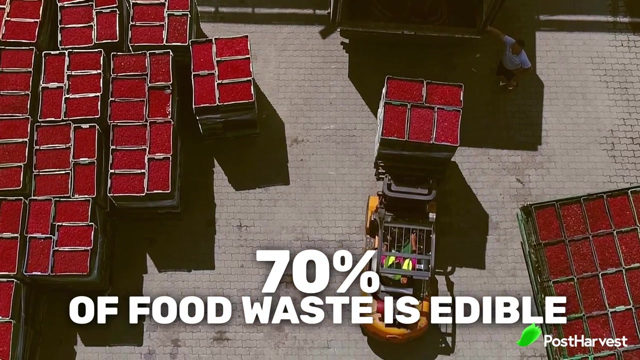 Number 10,: due to the unfavorable conditions inside landfills, it takes 25 years for a full hectare of lettuce to decompose. Number 11, around 70 percent of all global food waste is made up of uneaten food that is perfectly edible. Number 12,: 1.4 billion hectares of. 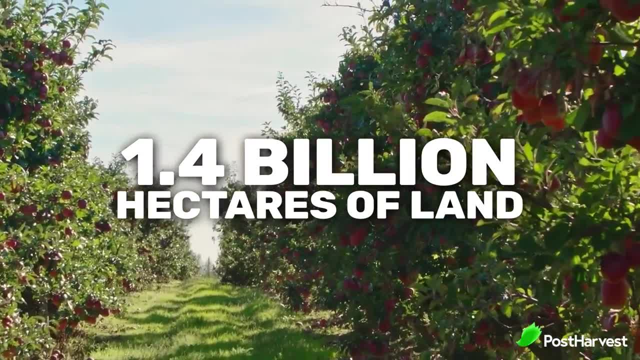 land is being used to grow global food products that will never be eaten. each year, That stretch of land is equal to the size of India, the European Union and the United States Number 10,. due to the unfavorable conditions inside landfills, it takes 25 years for a full hectare. 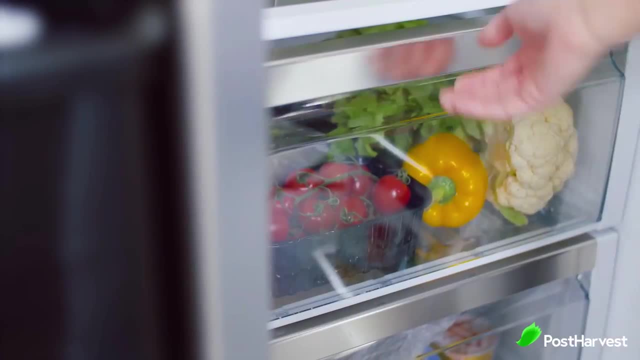 of lettuce to decompose That stretch of landfills. it takes 25 years for a full hectare of landfills, that stretch of landfills. it takes 25 years for a full hectare of lettuce to decompose. Number 13,: lack of education and awareness of simple things such as basic. 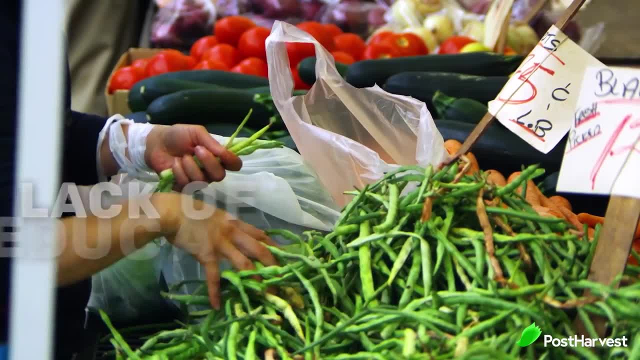 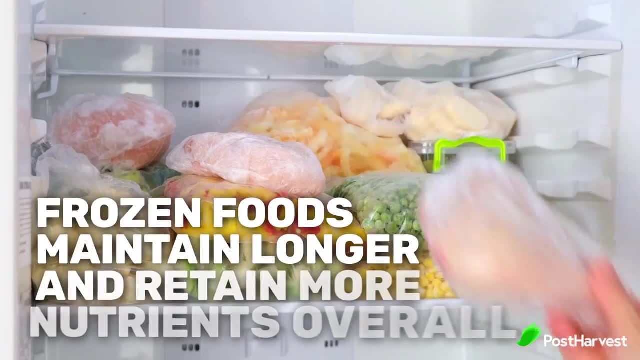 nutrition actually leads to further food waste amongst consumers. For example, many people believe that it is better to buy fresh food for quality and nutrients, but actually frozen foods maintain longer and retain more nutrients. overall Number 14, at the retail level, the 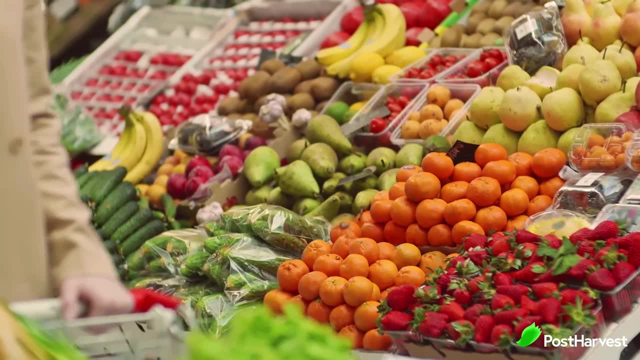 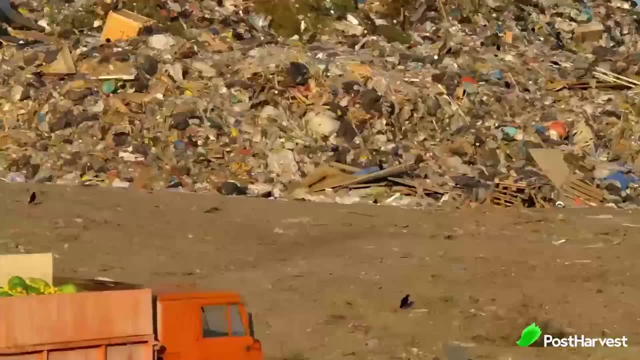 top global food waste issues are a result of a lack of thorough training, faulty equipment, ineffective processes and much more. Number 15, low-quality food concerning food and and over-ordering from distributors, resulting in a food surplus. And, finally, number 15.. 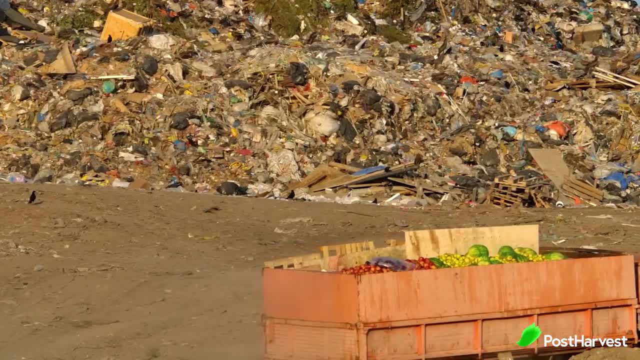 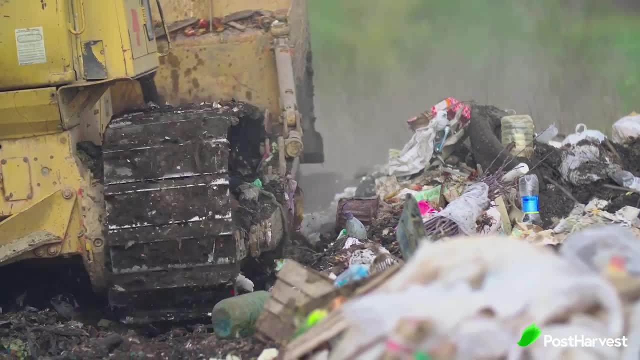 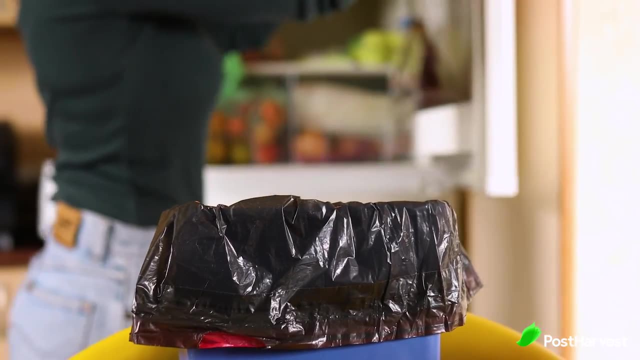 Food loss and waste items account for the largest percentage of materials found within landfills, accounting for 24.1% of all municipal solid waste. In summary, these numbers show the complexity and severity of food loss and waste Saving food is an imperative piece of creating a sustainable food future.